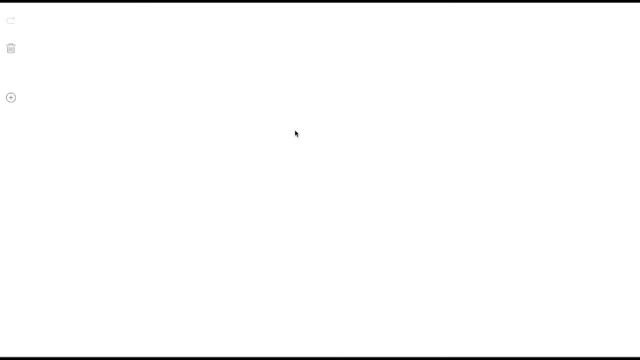 Implemented now, Like we are given a, b, c as string, a, b and c and we have the matrix which of size is greater than the type. text1 cross the size greater than 1 with size 2.. Okay, so if we say that the length of this string is n, 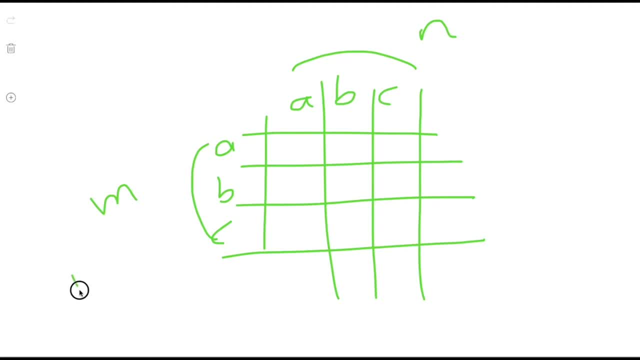 And string is m, then the size of the matrix should be n plus 1, cross m plus 1. ok, and in those the initial value would be 0 for all and a and a is equal. so take this value plus add with this 1, so it would be coming to be 1. a and b is not equal. if not equal, then take. 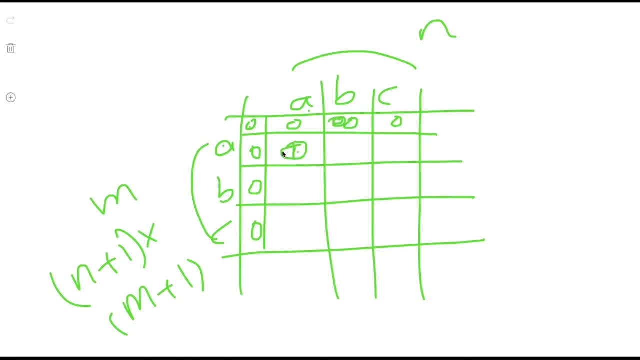 max of this value and this value, so it will be coming to be 1 and now this, and these are not equal. so take the max value of this both, which is 1 right now. this b and this a are also not equal, so take the max value from here and here, which is 1 now this b is equal. 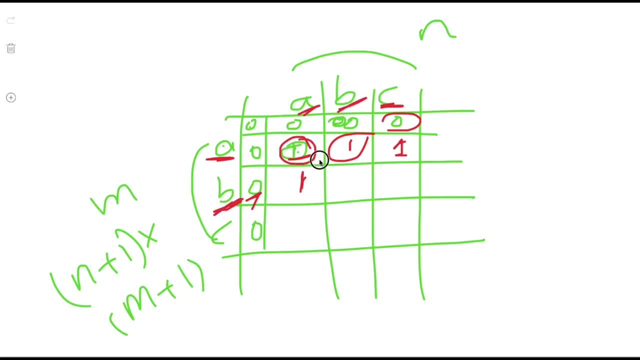 to this b, so take this value, add 1 to it, So the length would become 2 and follow on like this, so 2 would be coming here. 1, 1, c is not equal. 1 will be coming, c and b not equal, so 2 would be coming. c and c, this, c and this. 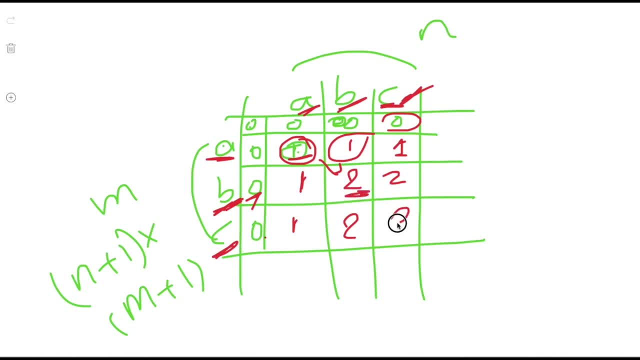 c. both are equal, so take this element plus add 1, so 3, and our solution lies at this place. that is dp of n, m, n. is the solution in this case? Right, that is length of first string and length of second string. ok, so it would be dp of n. 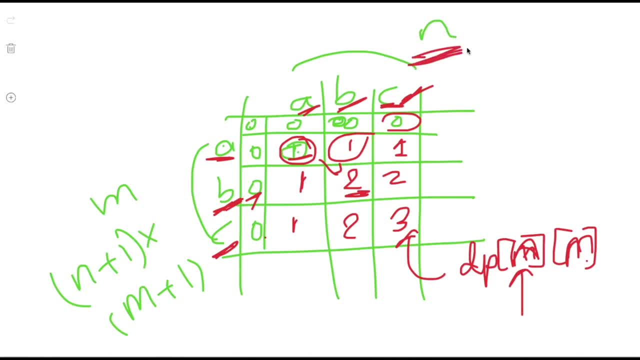 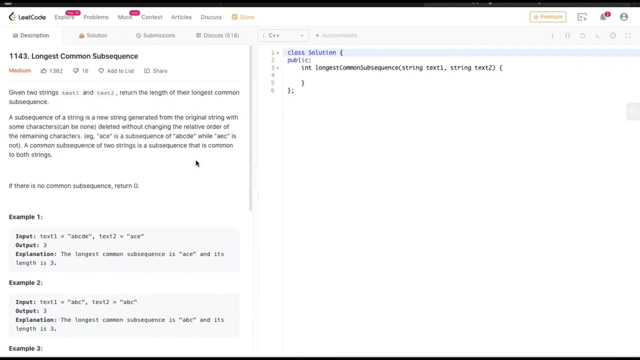 m, as we are considering this as a first string and this as a second string. ok, So let us implement this now and write a code. so the problem is this, which I have already written just now: text1 and text2 are given, which is in input, like they are providing. 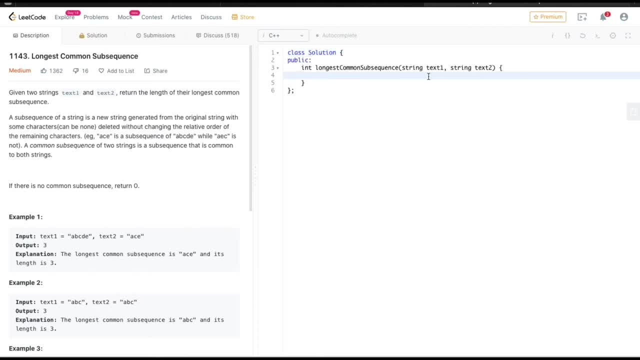 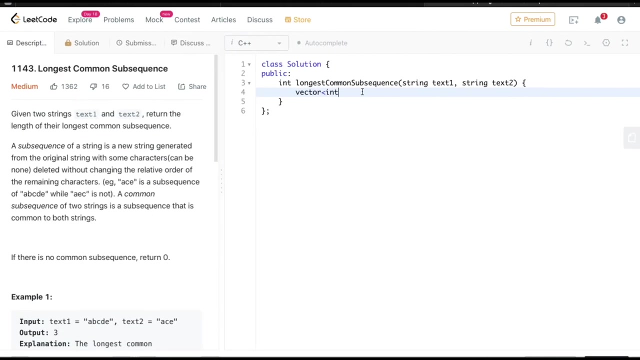 us with the input now. first let us make the two dimensional array named dp, of size: text1 dot size plus 1 and text2 dot size plus 1. so let us create dp. this i should be text1 dot size plus 1 comma, dp, not dp vector. text2- dot size plus. 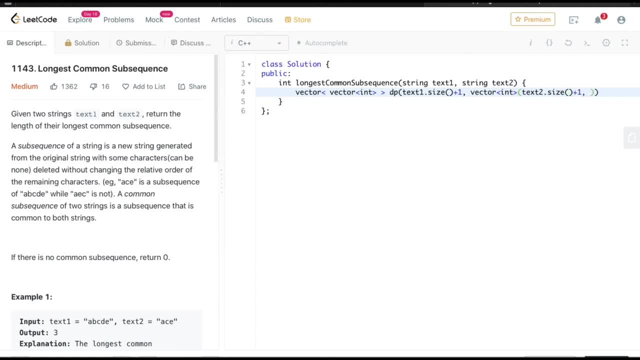 1 and initialize all the value to be 0 so that for first row and first column it will be so. for the first row and the first column the value would be pre filled and it should be filled with 0 right after that. for int: i equal to 1. i less than equal to text, i less. 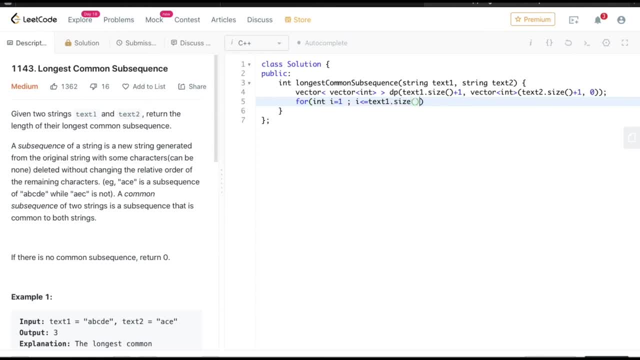 than equal to text, 1 dot size, i plus plus. so with this we will be traversing the first array and the index of array starts from 0. so we will be using i minus 1 and j minus 1 for the comparison purpose to traverse the second string. for int: j equal to 1, j less than equal to text. 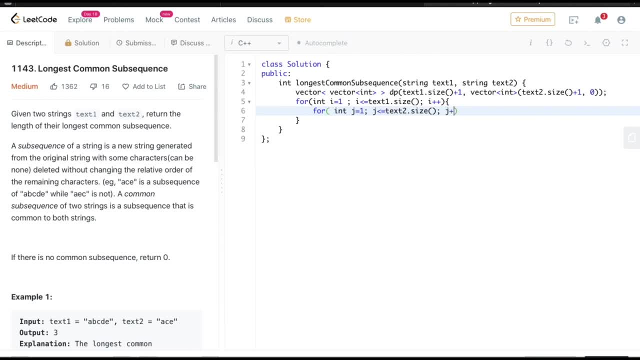 1 dot size j plus plus. now we need to apply the condition that when text1 is text1 and text2 are equal, then what we have to do and if not equal, then what we have to do. so if text1 dot i minus 1 is equal to text2 j minus 1, and if not equal, then what we have to do. 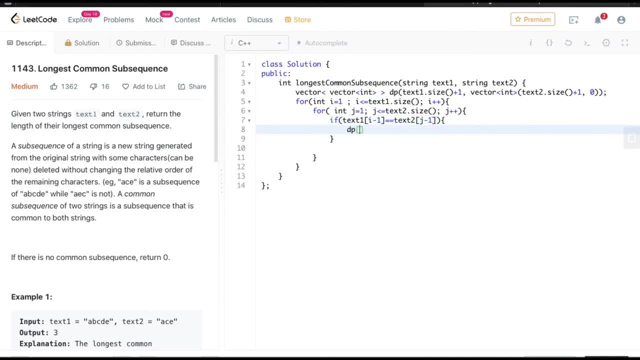 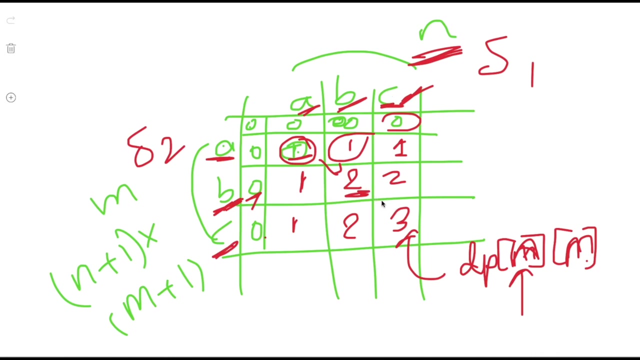 is if both are equal, then dp of i- j is equal to dp of i minus 1, j minus 1 plus 1, as we have seen here. like if c and c are equal, then we need to take this element, element's value and add for this value, right. 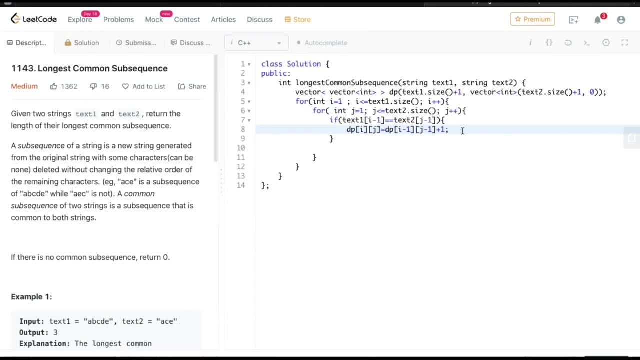 2 plus 1 would be 3 and in else condition, else dp of i j will be equal to max of dp of i minus 1, j comma dp of i j minus 1, and these two are the value which we are taking from this. 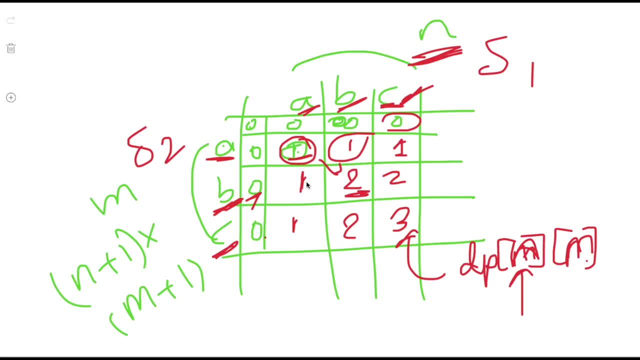 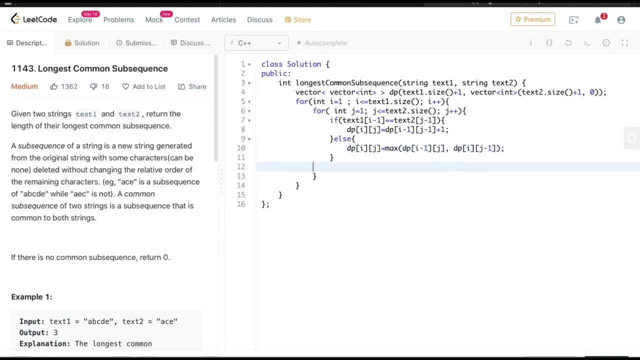 place, like if we see here, then b and a are not equal, so we need to take the max values from this place and this place. so this is getting done in the else condition, which is here right, and our solution lies at dp of text1.size and text2.size. so return dp, text1.size and text2.size as we. 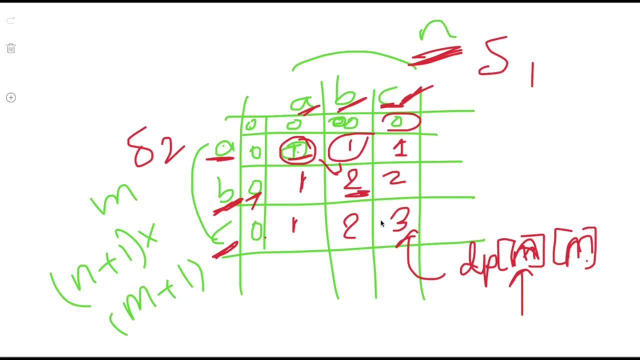 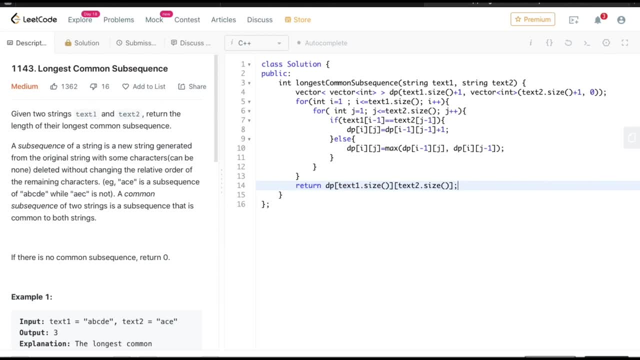 did here. our solution lies at the last position, so this is our answer, which we will be returning. so let's run the code. okay, so for a, b, c, d, e, a, c, e, two are the inputs, output should be three and we are also expected values, also three. so this is correct. and check it once again so that there should not be a.